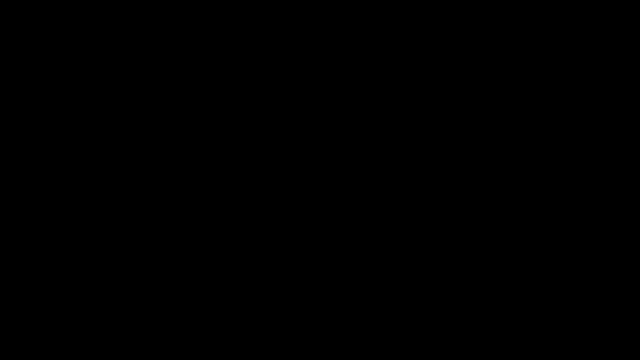 In this lesson we're going to talk about adding and subtracting rational expressions. What is 4 root 5 plus 6 root 5?? What is that? equal to Now, because the radicals are the same. you can add the coefficient in front of it, That is, you can add 4 plus 6, which? 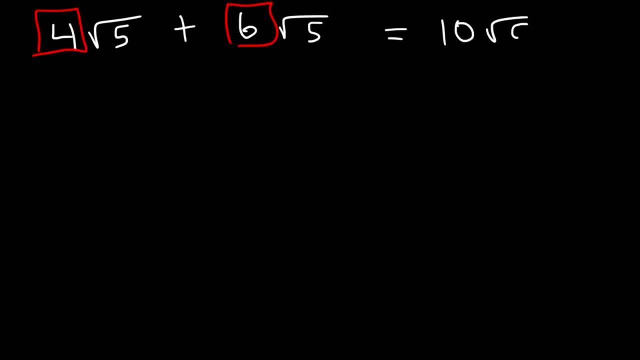 is 10.. So this is equal to 10 root 5.. Let's say, if you have 4 radical 3 plus 6 radical 5. You cannot add 4 plus 6, because what would you do? Would you say it's 10 root 3 or 10? 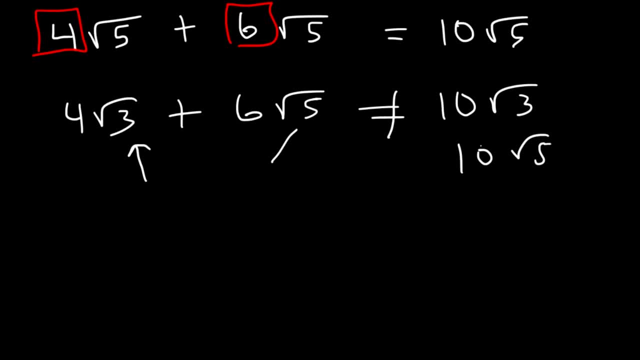 root 5?? It doesn't work, because these two are not the same. You can only add them if they're the same. For example, you can add 4x plus 6x, that's 10x, because they're like. 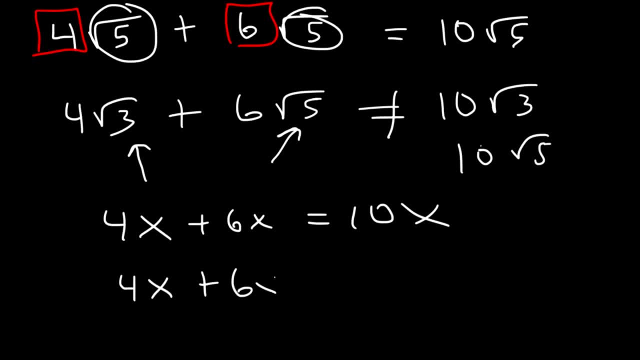 terms. But you can't add 4x plus 6x, because they're like terms. You can't say: 4x plus 6y is 10xy. It just doesn't work. See, you only can add or subtract. 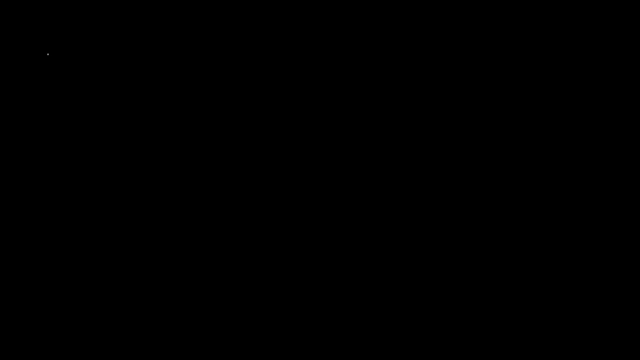 like terms. So, knowing that, go ahead and simplify this problem: 7 root 2 minus 3 root 2 plus 5 root 2.. So all of these are like terms. They all contain the square root of 2.. 7 minus 3 is 4, and 4 plus 5 is 9.. 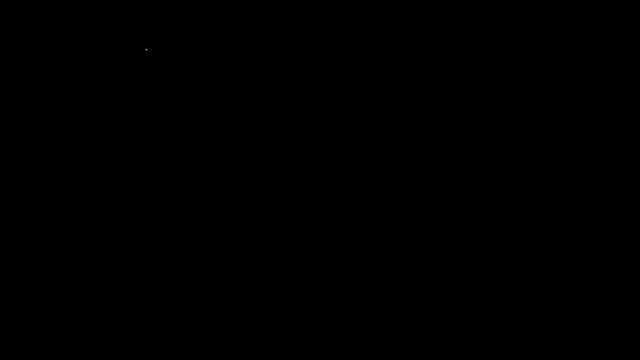 So it's 9 root 2.. Now, what about this one? What's 3 times the square root of 8 minus 5 times the square root of 18?? Right now we cannot combine them, because 8 and 18 are. 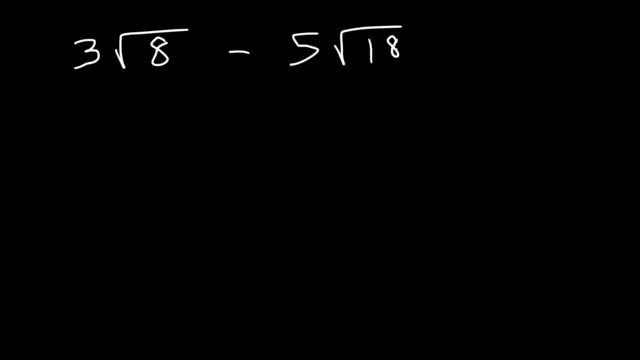 not the same, But sometimes we can simplify the radicals and make it the same. 8 is basically 4 times 2.. 9 times 2.. The square root of 4 is 2, and the square root of 9 is 3.. 3 times 2 is 6.. 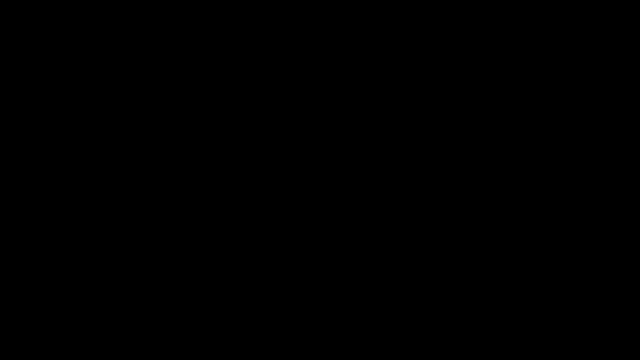 In this lesson we're going to talk about adding and subtracting rational expressions. What is 4 root 5 plus 6 root 5?? What is that? equal to Now, because the radicals are the same. you can add the coefficient in front of it, That is, you can add 4 plus 6, which? 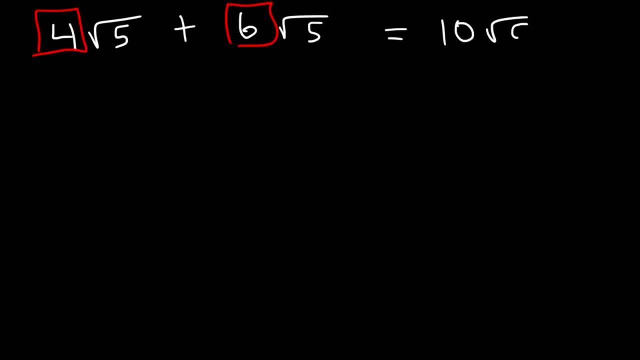 is 10.. So this is equal to 10 root 5.. Let's say, if you have 4 radical 3 plus 6 radical 5. You cannot add 4 plus 6, because what would you do? Would you say it's 10 root 3 or 10? 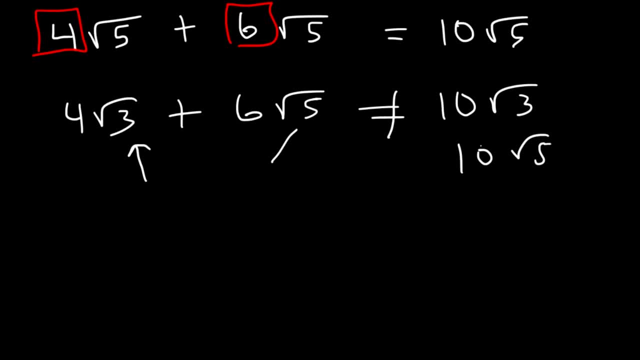 root 5?? It doesn't work, because these two are not the same. You can only add them if they're the same. For example, you can add 4x plus 6x, that's 10x, because they're like. 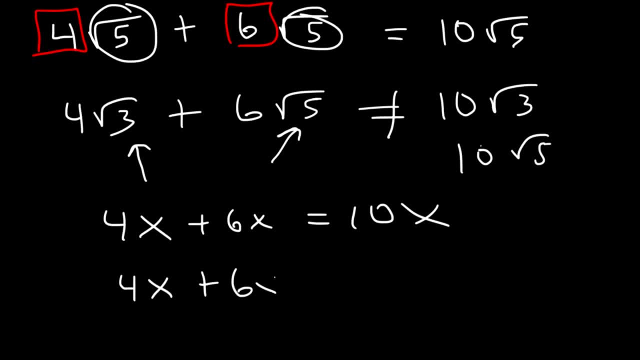 terms. But you can't add 4x plus 6x, because they're like terms. You can't say: 4x plus 6y is 10xy. It just doesn't work. See, you only can add or subtract. 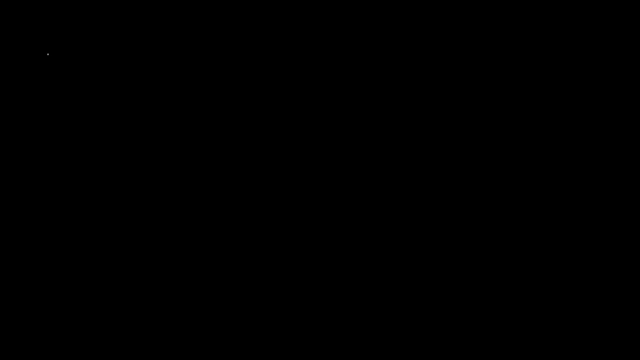 like terms. So, knowing that, go ahead and simplify this problem: 7 root 2 minus 3 root 2 plus 5 root 2.. So all of these are like terms. They all contain the square root of 2.. 7 minus 3 is 4, and 4 plus 5 is 9.. 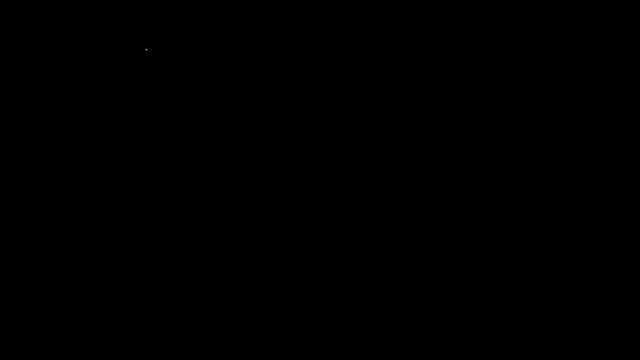 So it's 9 root 2.. Now, what about this one? What's 3 times the square root of 8 minus 5 times the square root of 18?? Right now we cannot combine them, because 8 and 18 are. 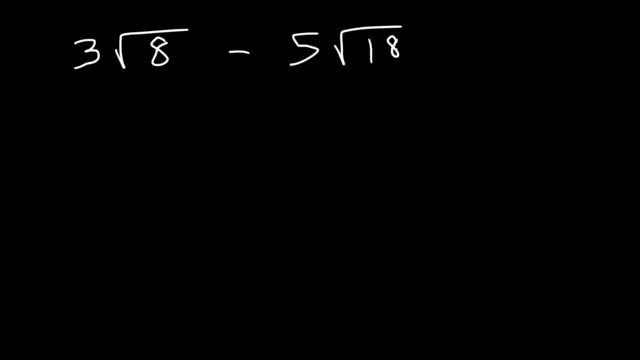 not the same, But sometimes we can simplify the radicals and make it the same. 8 is basically 4 times 2.. 9 times 2.. The square root of 4 is 2, and the square root of 9 is 3.. 3 times 2 is 6.. 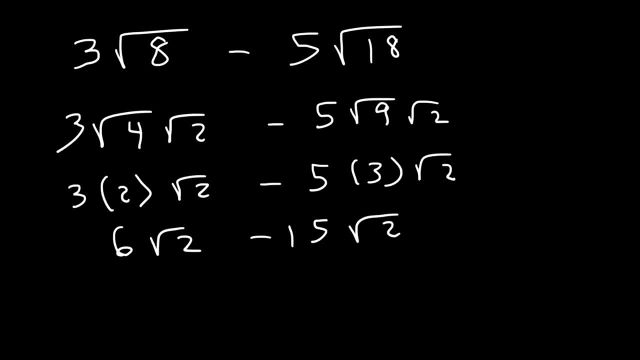 5 times 3 is 15.. Now notice that we have like terms, So now we can combine them: 6 minus 15 is negative 9.. So the final answer is negative 9 root. 2.. Try this one: 4 root. 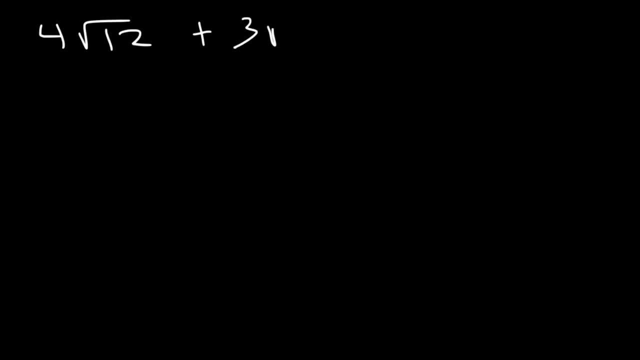 12 plus 3 root 27 minus 2 root 48.. Feel free to pause the video and work on this example. So 12, we can break that into 4 and 3.. 27,. the perfect square that goes into 27 is 9.. 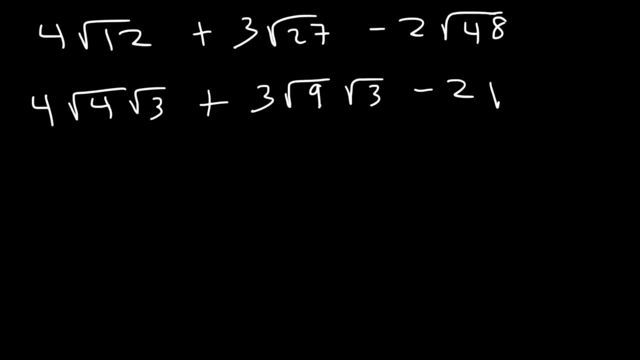 So 9 and 3. And 48 contains the perfect square, which is 16.. Notice that we have a common radical root: 3.. So we're on the right track. The square root of 4 is 2. The square. 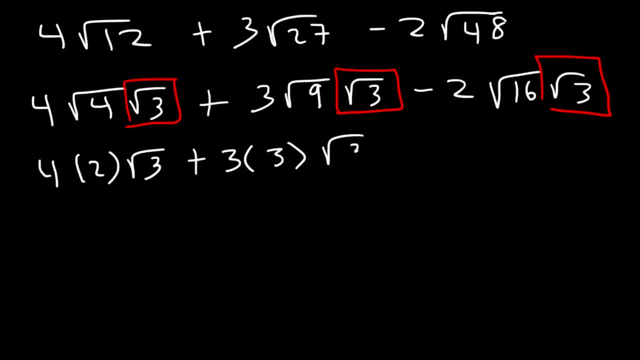 root of 9 is 3. And the square root of 16 is 4.. 4 times 2 is 8.. 3 times 3 is 9.. 2 times 4 is 8.. So 8 and negative 8, they cancel, They add up to 0.. So the final answer is: 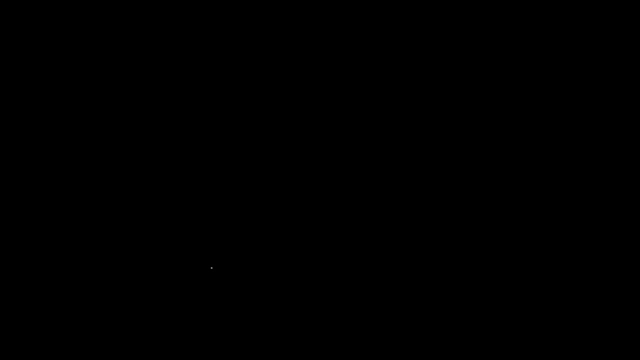 just going to be 9 plus 3.. So we're on the right track. We're on the right track. So 9 root 3.. Let's try one more example, but this time we're going to use cube roots. 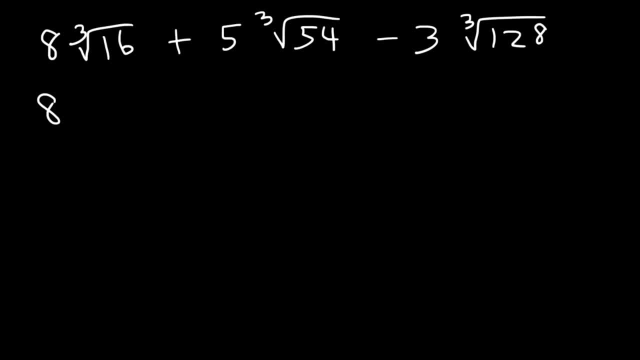 Go ahead and try that. So think of the perfect cubes: 8,, 27,, 64,, 125.. 8 goes into 16.. So you want to break down 16 as 8 and 2.. 27 goes into 54. So 54 divided by 27 is 2.. 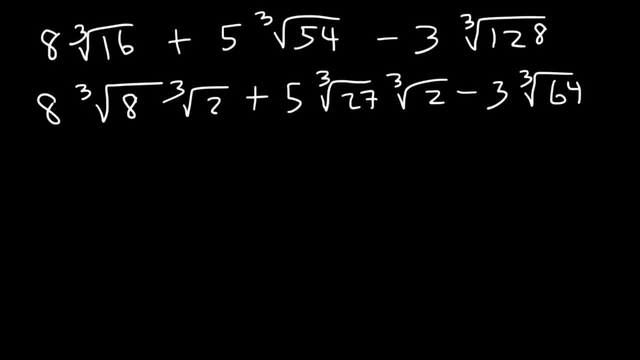 And 64 goes into 128.. 64 times 2 is 128.. Notice that every term has a cube root of 2.. So these are all like terms. The cube root of 8 can be simplified to 2.. And the. 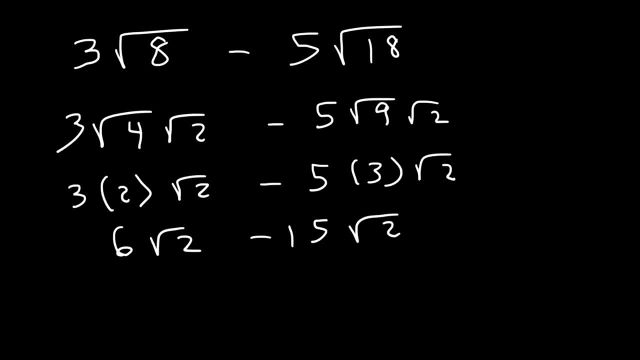 5 times 3 is 15.. Now notice that we have like terms, So now we can combine them: 6 minus 15 is negative 9.. So the final answer is negative 9 root. 2.. Try this one: 4 root. 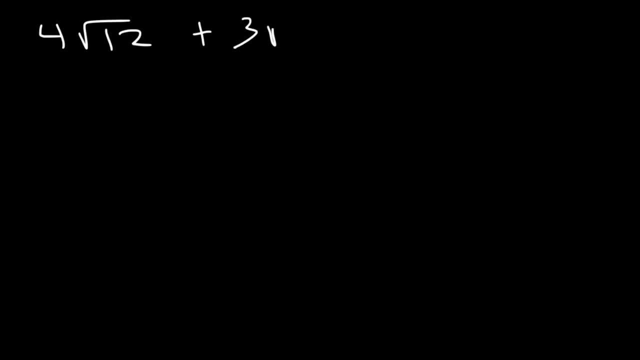 12 plus 3 root 27 minus 2 root 48.. Feel free to pause the video and work on this example. So 12, we can break that into 4 and 3.. 27,. the perfect square that goes into 27 is 9.. 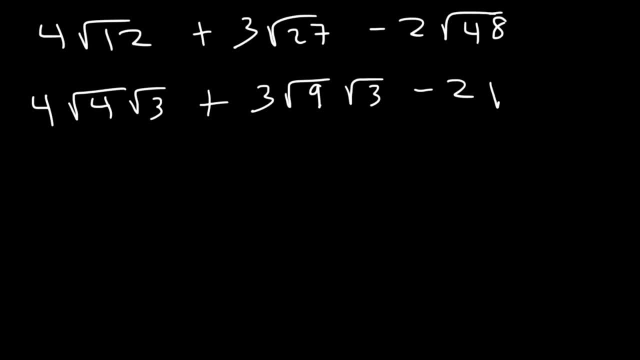 So 9 and 3.. And 48 contains the perfect square, which is 16.. Notice that we have a common radical root: 3.. So we're on the right track. The square root of 4 is 2.. The 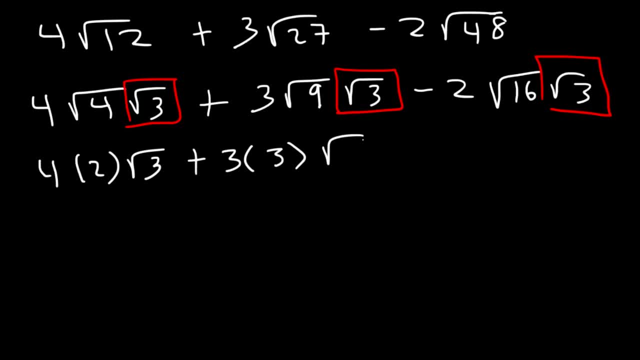 square root of 9 is 3. And the square root of 16 is 4.. 4 times 2 is 8.. 3 times 3 is 9.. 2 times 4 is 8.. So 8 and negative 8.. They cancel, They add up to 0.. So the final answer: 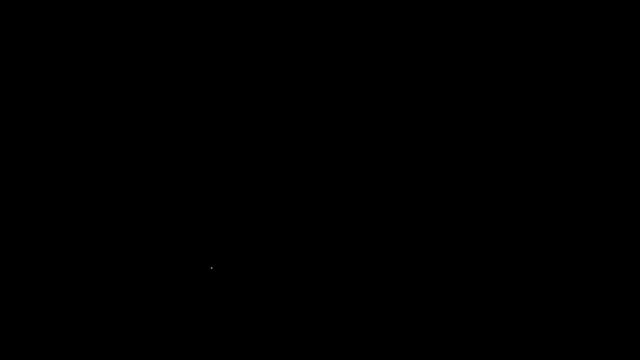 is just going to be 9…. Let's try one more example, but this time we're going to use cube roots. Go ahead and try that. So think of the perfect cubes: 8,, 27,, 64, and 125,. 8 goes into 16,. so you want to break? 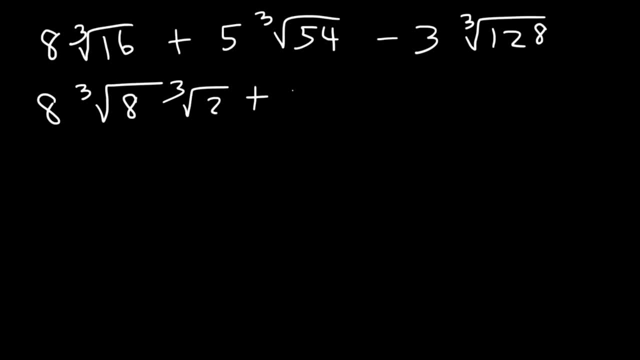 down 16 as 8 and 2.. 27 goes into 54, so 54 divided by 27 is 2, and 64 goes into 128,. 64 times 2 is 128.. Notice that every term has a cube root of 2, so these are all like terms. 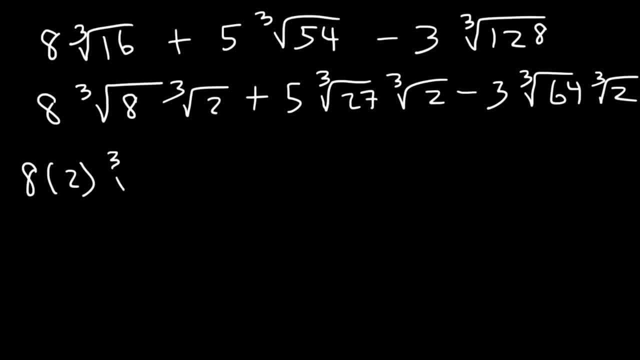 The cube root of 8 can be simplified to 2, and the cube root of 27 is 3, and the cube root of 64 is 4.. So 8 times 2 is 16,, 5 times 3 is 15, and 3 times 4 is 12.. 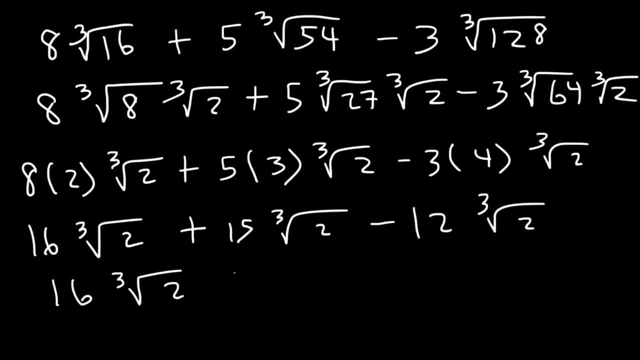 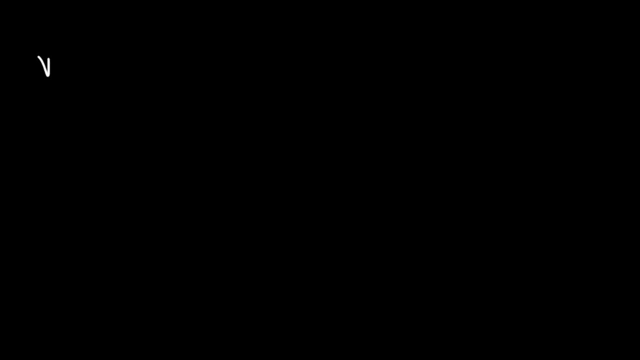 Now 15 minus 12 is 3. And 16 plus 3 is 19,. so the answer is 19 cube root 2.. If you were to see a homework problem that looks like this, what would you do? What is the square root of 3 times 7 plus root 3?? 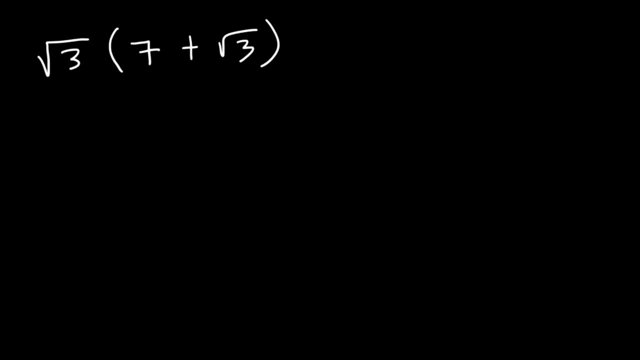 Feel free to try that problem. So here you have to distribute: Root 3 times 7 is simply 7 root 3.. So what would you do? What would you do? You would divide root 3, and root 3 times itself. 3 times 3 is 9,, so that's the square. 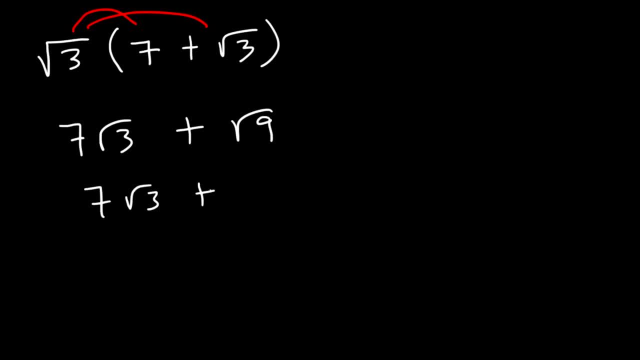 root of 9, and the square root of 9 is 3.. So that's the answer You just got to distribute. Try this one: What is 4 root, 5 times root, 7, minus the square root of 3?? 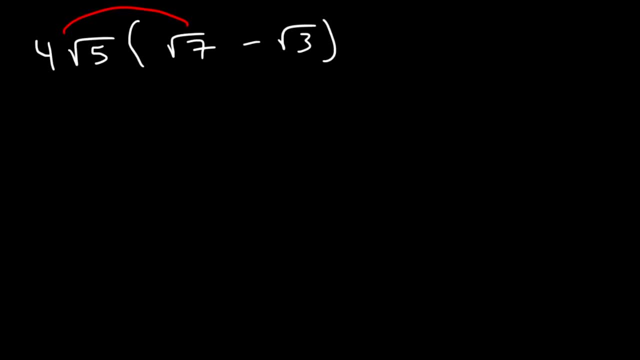 Feel free to pause the video and work on that example. So let's multiply the first two. We can't multiply 4 and 7 because the 7 is inside the radical And the 4 is on the outside. However, we can multiply 5 and 7 because they're both inside the square root function. 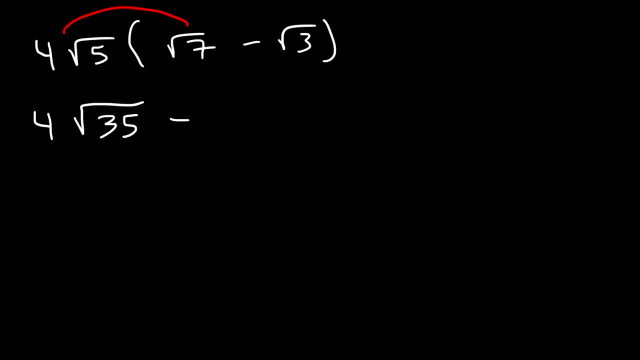 5 times 7 is 35. And then let's multiply 4 root 5 by root 3.. So 5 times 3 is 15. And that's going to be inside the radical, And so that's the answer. 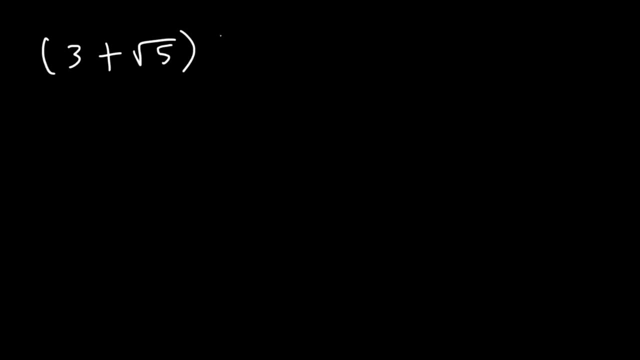 Now, sometimes you might be given a problem where you have to multiply two conjugates, Okay, Two conjugates together. Whenever you see this, you need to FOIL and know that the middle terms will cancel. So first, it's going to be 3 times 3, which is 9.. 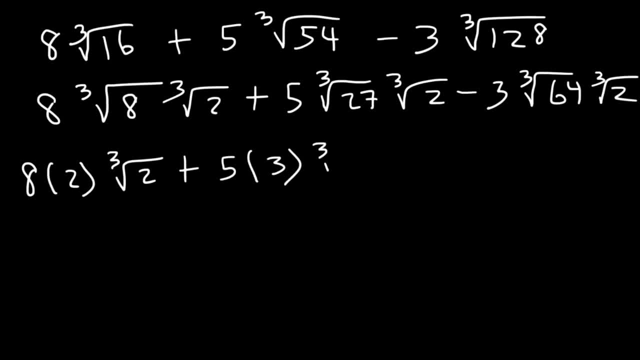 cube root of 27 is 0.. So we're on the left track And now we're going to find out what's the perfect square. 3, and the cube root of 64 is 4.. So 8 times 2 is 16,, 5 times 3 is 15, and 3. 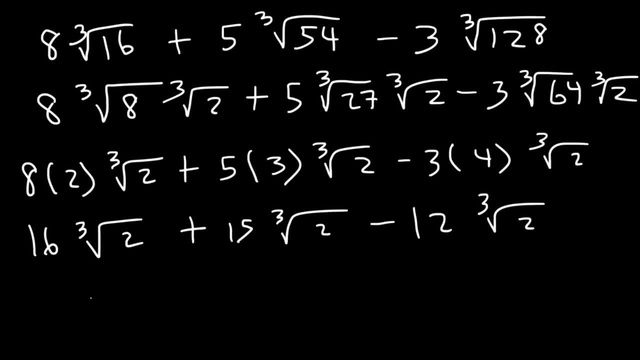 times 4 is 12.. Now 15 minus 12 is 3, and 16 plus 3 is 19.. So the answer is 19 cube root 2.. If you were to see a homework problem that looks like this, what would 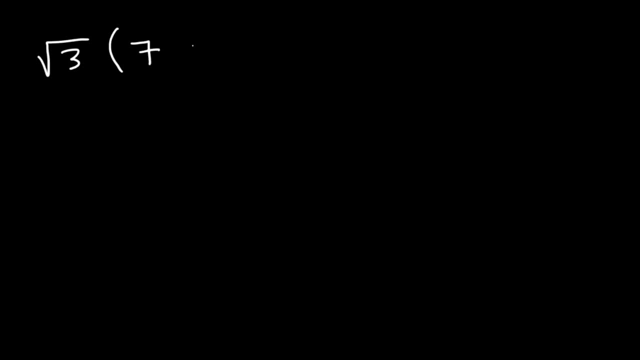 you do? What is the square root of 3 times 7 plus root 3?? Feel free to try that problem. So here you have to distribute: Root 3 times 7 is simply 7, root 3, and root 3 times itself. 3 times 3 is 9,, so that's the square root of 9.. 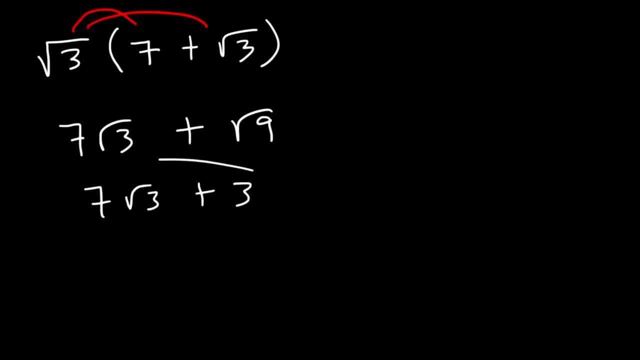 And the square root of 9 is 3.. So that's the answer You just got to distribute. Try this one: What is 4 root 5 times root 7 minus the square root of 3?? Feel free to pause the video and work on that example. So let's multiply the first two. 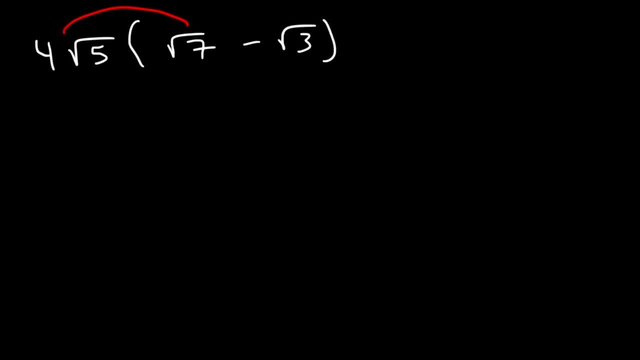 We can't multiply 4 and 7 because the 7 is inside the radical and the 4 is on the outside. However, we can multiply 5 and 7 because they're both inside the square root function. 5 times 7 is 35.. And then let's multiply 4 root 5 by root 3.. So 5 times 3 is 15, and 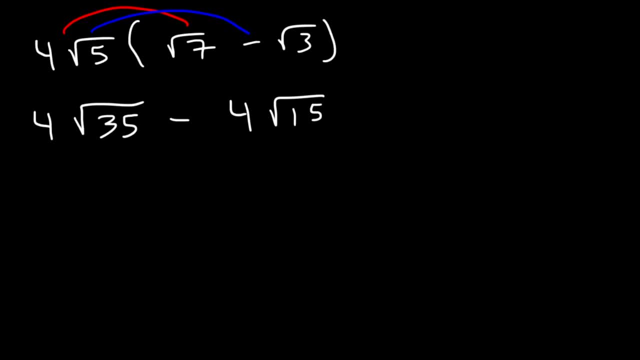 that's going to be inside the radical, And so that's the answer. Now, sometimes you might be given a problem where you have to multiply two conjugates together. Whenever you see this, you need to FOIL and know that the middle terms will cancel. 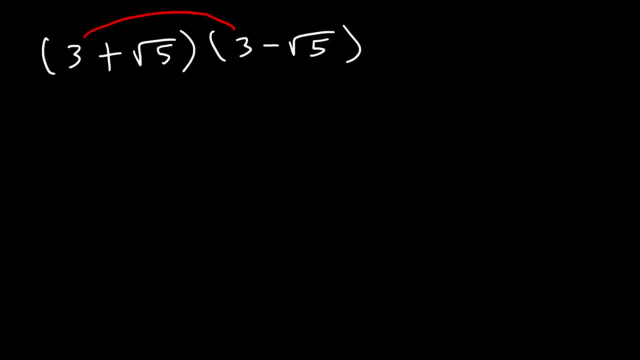 So first it's going to be 3 times 3,, which is 9.. And then we're going to multiply 3 times negative root 5.. That's negative 3 root 5.. And then root 5 times 3.. So that's positive 3 root 5.. And the square root of 5 times negative root 5.. 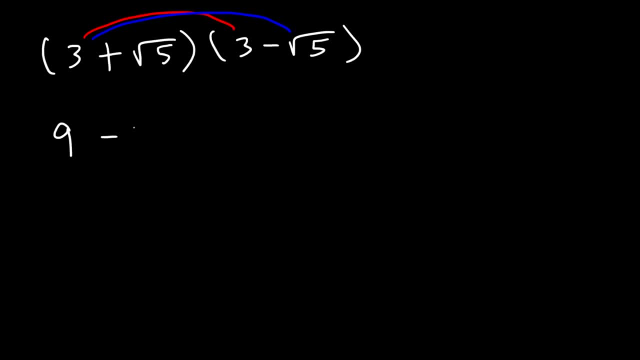 And then we're going to multiply 3 times negative root 5, that's negative 3 root 5.. And then root 5 times 3,, so that's positive 3 root 5.. And the square root of 5 times negative root 5.. 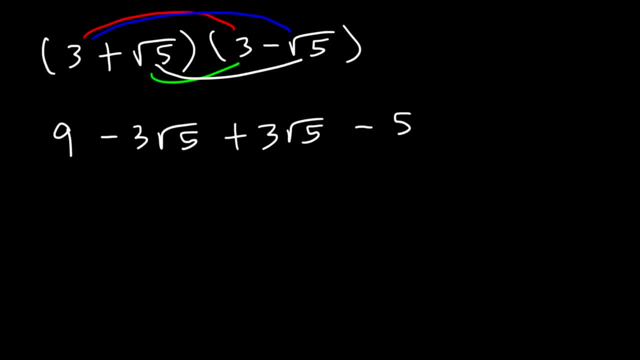 That's negative root 25, which is negative 5.. The two middle terms will cancel. they add up to 0.. And 9 minus 5 is equal to 4.. Let's try another example: 4 minus root, 6 times 4 plus root, 6.. 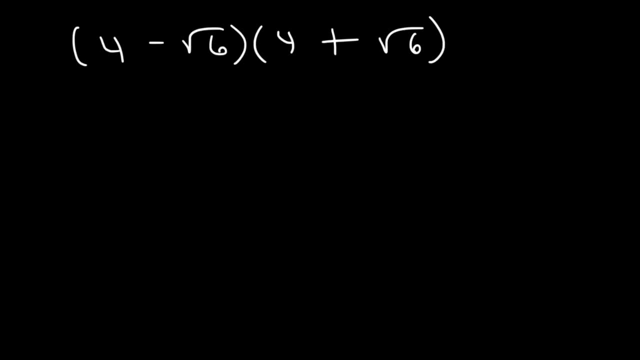 So we already know that the middle terms will cancel. So all we need to do is multiply the outer terms 4 times 4 is 16.. And negative root 6 is 15.. And negative root 6 times root 6.. 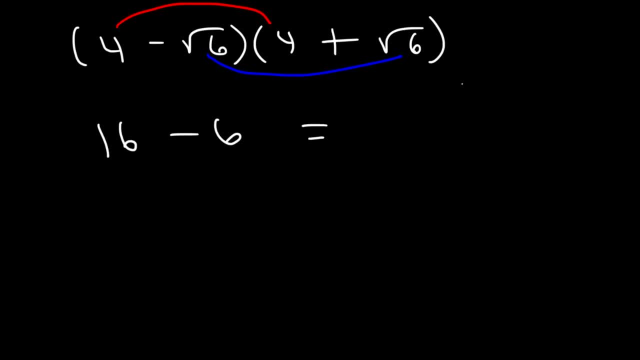 That's negative root 36,, which is negative 6.. And 16 minus 6 is 10.. That's going to be the final answer. Now, what about this one? What is 2 plus root 3 squared? If you see it, you need to expand it. 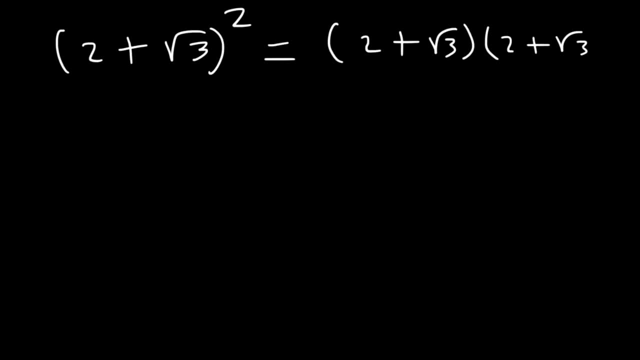 You have to multiply it by itself two times. Now, in this example these are not conjugates of each other because the sign is the same. Therefore the middle terms will not cancel. So we need to FOIL completely: 2 times 2 is 4.. 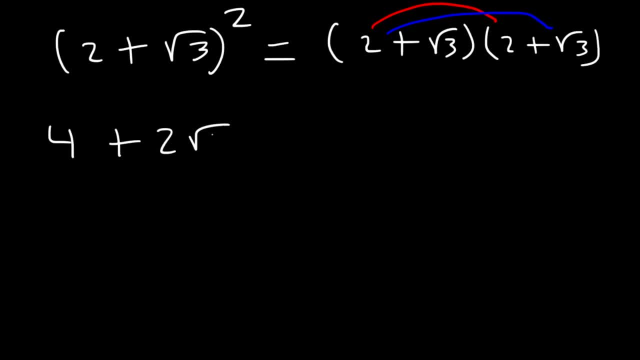 2 times root 3, that's positive 2 root 3.. And then root 3 times 2, that's also 2 root 3.. And root 3 times root 3 is just 3.. So let's add the middle terms. 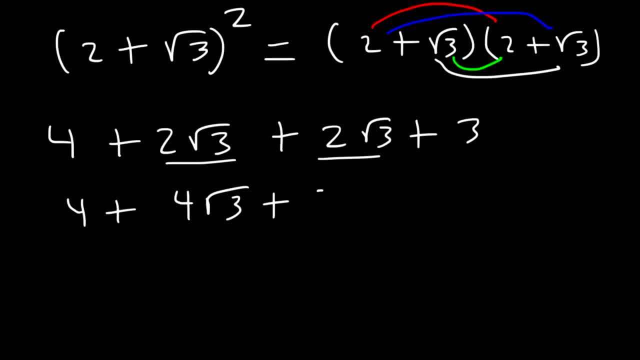 2 plus 2 is 4.. So that's going to be 4 root 3.. And 4 plus 3 is 7.. So that's going to be 4 root 3.. So it's 7 plus 4 root 3.. 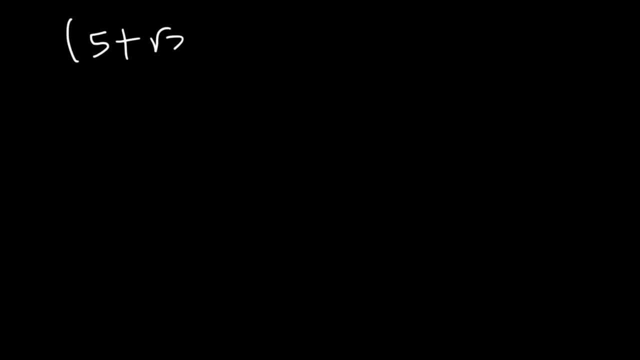 Let's try one more example: 5 plus root 2 squared, So 5 times 5, is 25.. We know the two middle terms will be 5 root 2.. And the last one, that's simply going to be 2.. 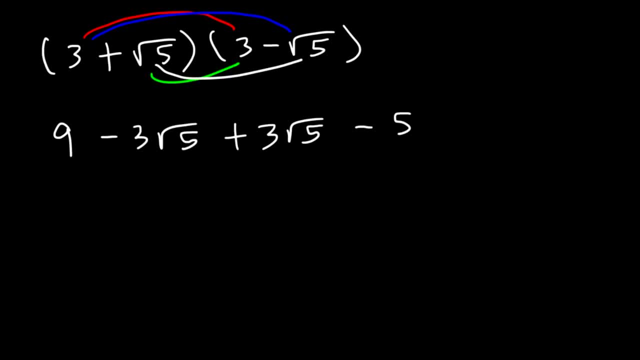 That's negative root 25, which is negative 5.. The two middle terms will cancel. They add up to 0.. And 9 minus 5 is equal to 5.. Let's try another example: 4 minus root, 6 times 4 plus root 6.. So we already know. 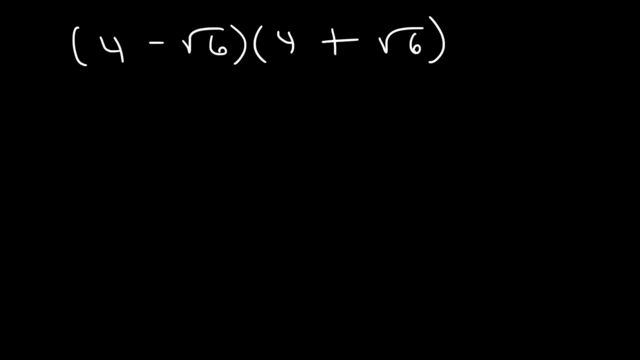 that the middle terms will cancel. So all we need to do is multiply the outer terms 4 times 4 is 16.. And negative root 6 times root 6.. That's negative root 36,, which is negative 6.. And 16 minus 6 is 10.. That's going to be the final answer. 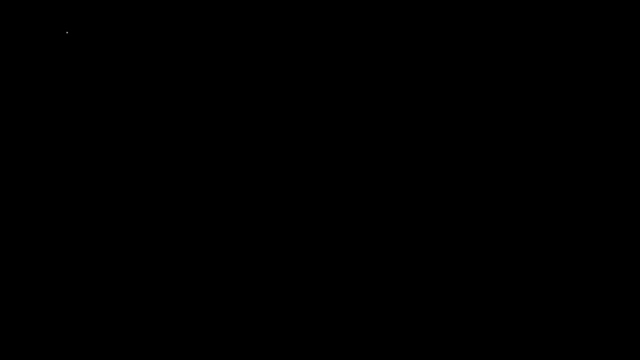 Now, what about this one? What is 2 plus root, 3 squared? If you see it, you need to expand it. You have to multiply it by itself two times. Now, in this example, these are not conjugates of each other, because the sign is the same. 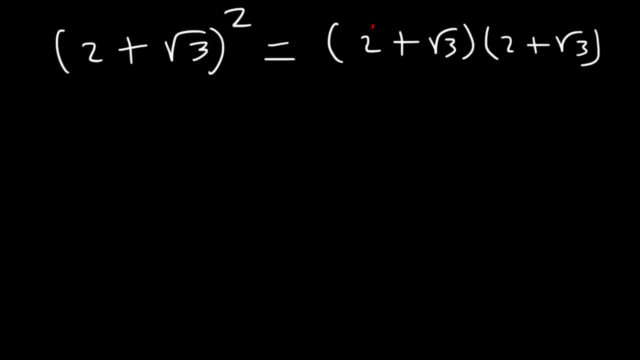 Therefore the middle terms will not cancel, So we need to FOIL completely: 2 times 2 is 4. 2 times root 3.. That's positive 4. 2 root 3, and then root 3 times 2, that's also 2 root 3, and root 3 times root 3 is. 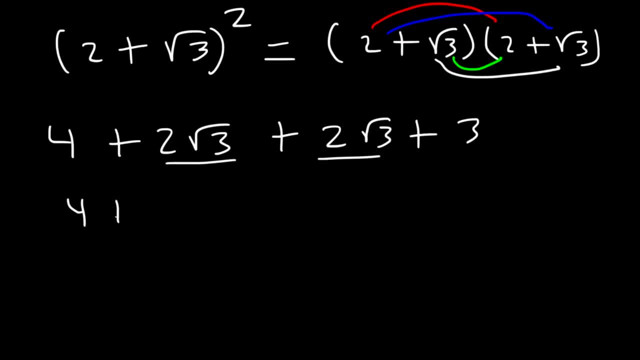 just 3.. So let's add the middle terms: 2 plus 2 is 4,, so that's going to be 4 root 3, and 4 plus 3 is 7,, so it's 7 plus 4 root 3.. Let's try one more example: 5 plus root 2. 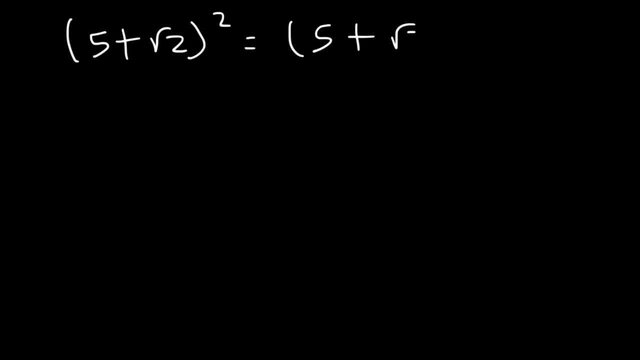 squared. So 5 times 5 is 25.. We know the two middle terms will be 5 root 2, and the last one that's simply going to be 2.. 5 plus 5 is 10, and 25 plus 2 is 27,, and so this is the answer. So here's another. 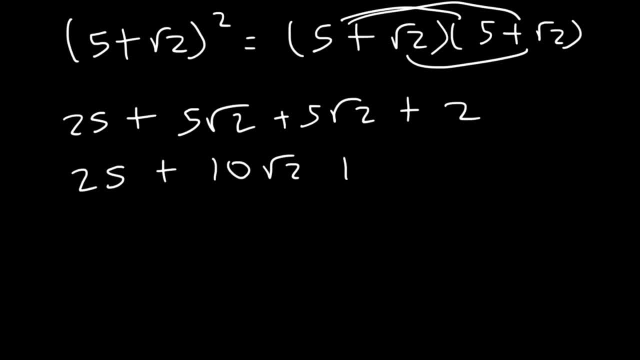 5 plus 5 is 10.. And 25 plus 2 is 27.. And so this is the answer. So here's another example that we can try, Go ahead and expand it and simplify. So 4 square root, 3 plus 2 raised to the third power. 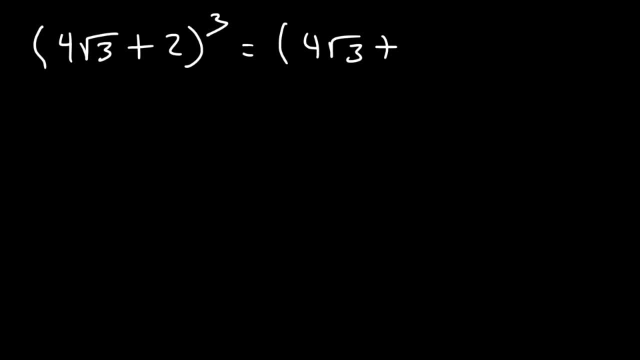 So we can write this three times 4, square root, 3 plus 2 raised to the third power. And I'm running out of space as always, But first let's FOIL the first two. So 4 times 4, that's 16.. 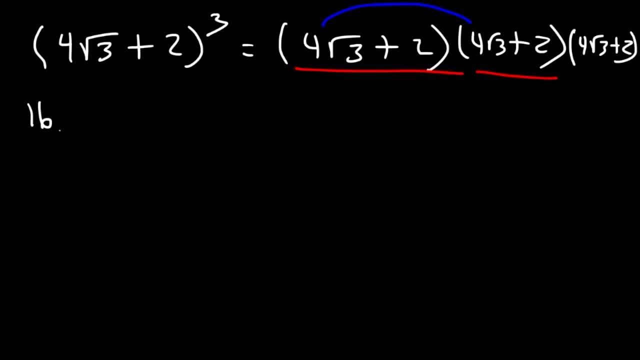 And the square root of 3 times the square root of 3, that's the square root of 9,, which is 3.. And then we have 4 times 2,, which is 8.. And the square root of 3 will be carried over. 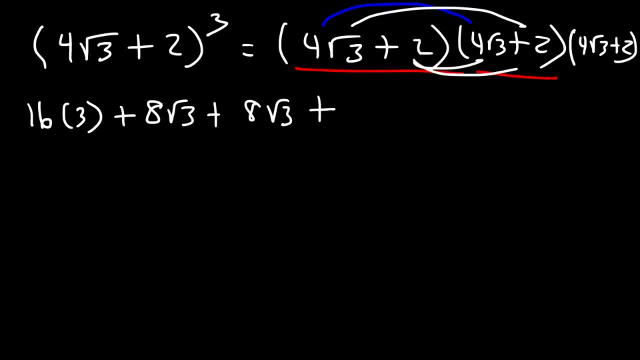 And this is also 8. So 8 square root 3. And then 2 times 2 is 4.. Now we still have another one that we're going to have to multiply later, But let's just write this for now. 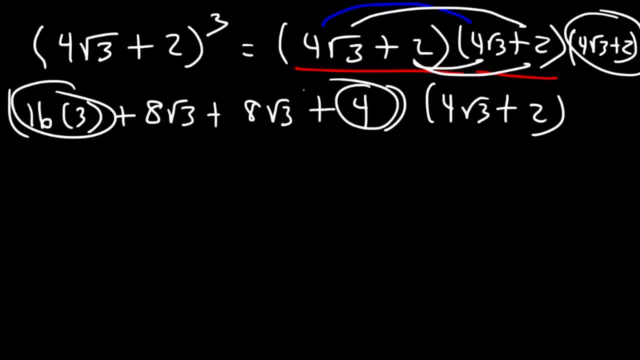 So 16 times 3 is 48.. 48 plus 4 is 52.. And 8 plus 8, that's 16.. So we've got 16 square root 3.. So now we need to FOIL these two expressions. 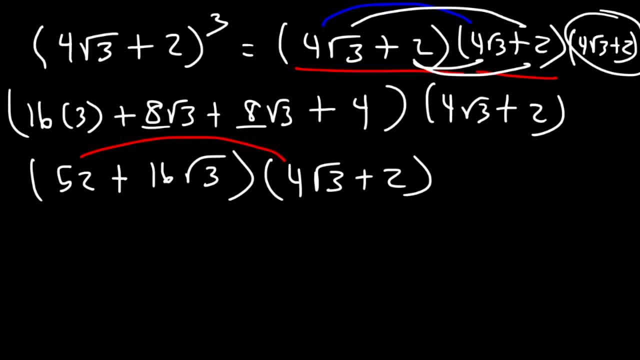 So now 52 times 4.. 50 times 4 is 200.. And 2 times 4 is 8.. So that's going to be 208, square root 3.. And then 52 times 2, that's 104.. 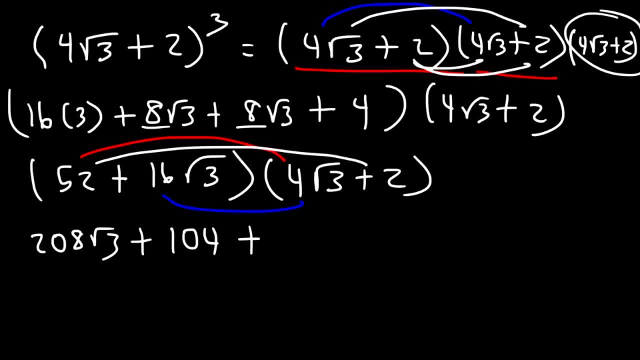 And here we have 16 times 4,, which is going to be 64.. And then square root 3 times square root 3, that's 3.. And then 16 times 2 is 32.. But it's going to be 32 square root 3.. 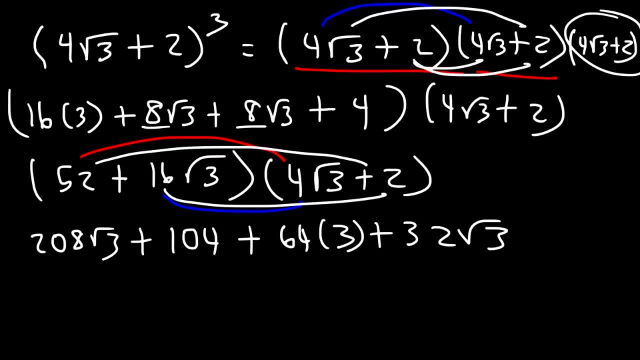 Now, 64 times 3 is 192.. If we add that to 104, that's 296.. And then we could add these two, So 208 plus 32, that's going to be 240.. So this is the final answer. 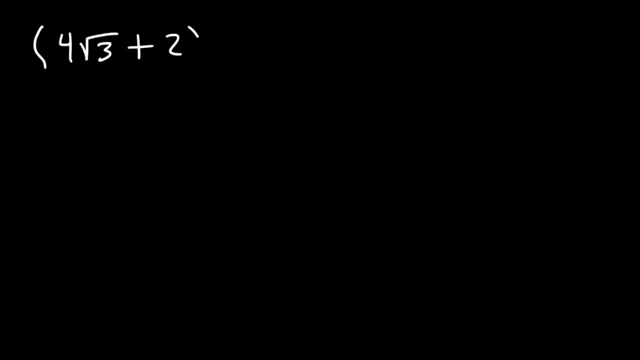 example, that we can try Go ahead and expand it and simplify. So 4 square root, 3 plus 2 raised to the third power. So we can write this three times, And I'm running out of space as always, But first let's FOIL the first two. So 4 times. 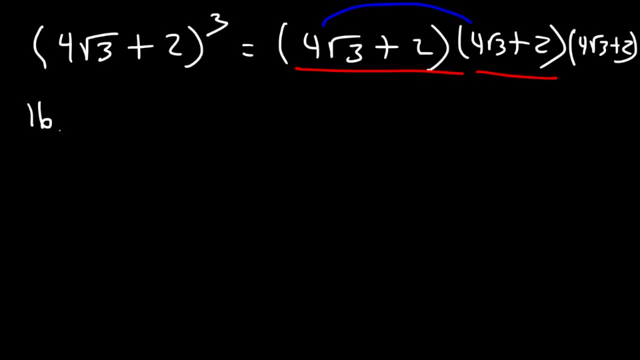 4,, that's 16.. And the square root of 3 times the square root of 3,, that's the square root of 9,, which is 3.. And then we have 4 times 2,, which is 8,, and the square root of 3 will. 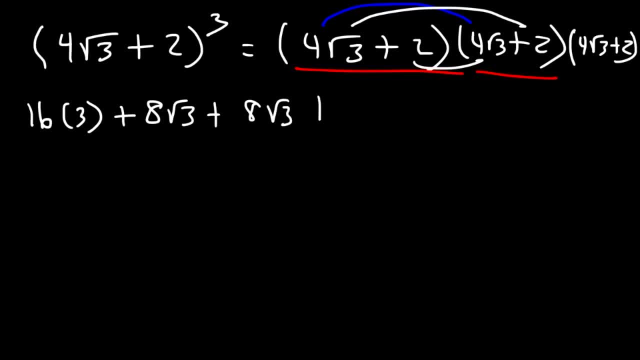 be carried over. This is also 8 square root 3, and then 2 times 2 is 4.. Now we still have another one that we're going to have to multiply later, but let's just write this for now. So 16 times 3 is 48.. 48 plus 4 is 52.. And 8 plus 8, that's 16.. So we've got 16 square. 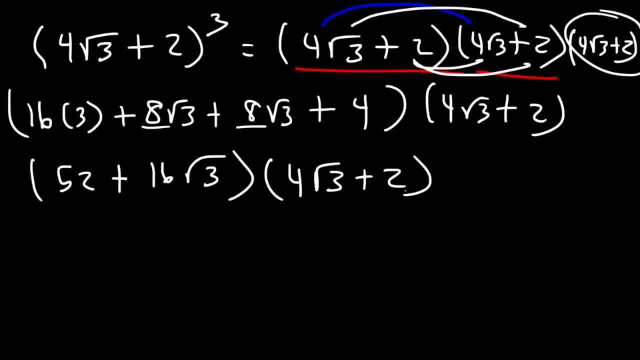 root 3.. So now we need to FOIL these two expressions. So now 52 times 4.. 50 times 4 is 200, and 2 times 4 is 8.. So that's going to be 208 square. 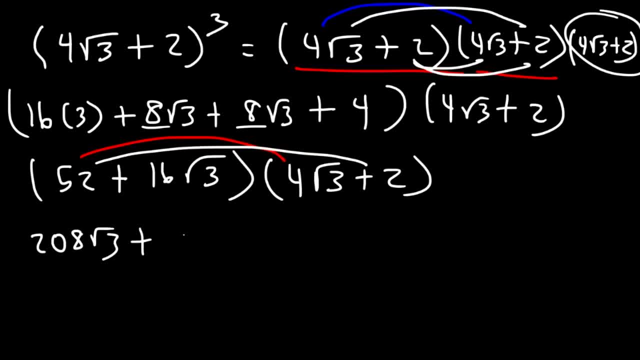 root 3.. And then 52 times 2, that's 104.. And here we have 16 times 4,, which is going to be 64.. And then square root 3 times square root 3, that's 3.. And then 16 times 2 is 32, but it's. 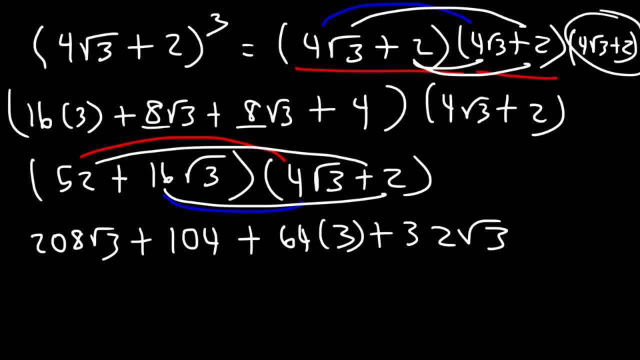 going to be 32 square root 3.. Now, 64 times 3 is 192.. If we add that to 104, that's 296.. And then we could add these two, So 208 plus 32, that's going to be 240.. 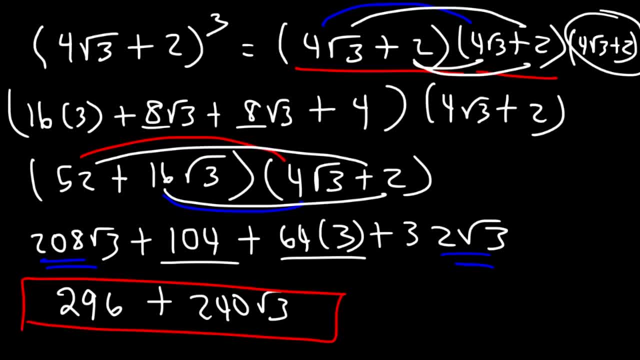 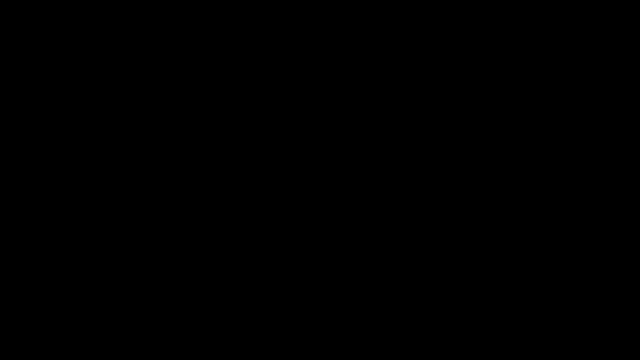 So this is the final answer: 296 plus 240 square root 3.. That's the final answer.